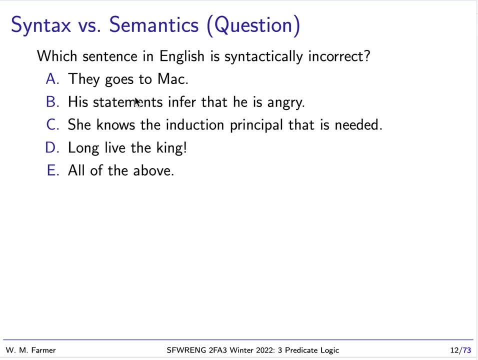 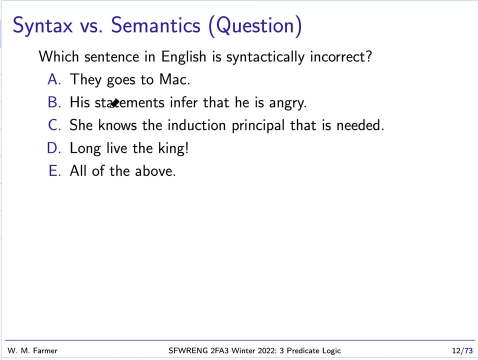 Okay, welcome back. It turns out that All of these sentences are syntactically correct, At least the first four, except for A. A should be, A should be. they go to Mac. B, C and D are syntactically correct, but semantically they are not correct. 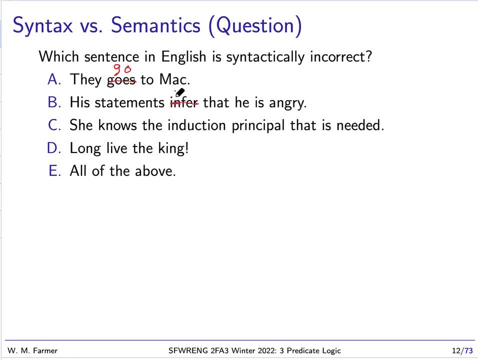 His statements infer that he is angry. No, He should say: his statements Imply that he is angry. She knows the induction principle that is needed. No, This should be principle. spelled like this: And long live the king. You might think that there should be long lives the king. 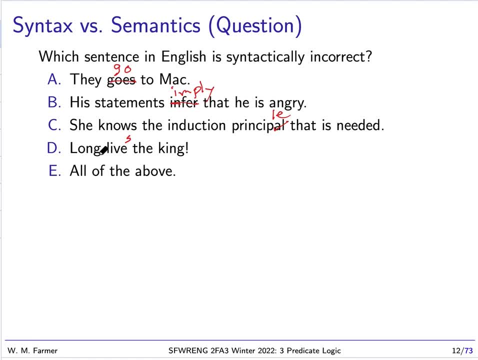 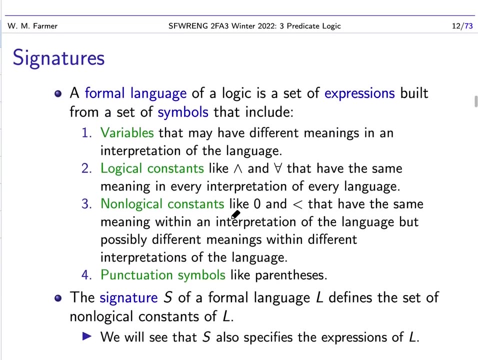 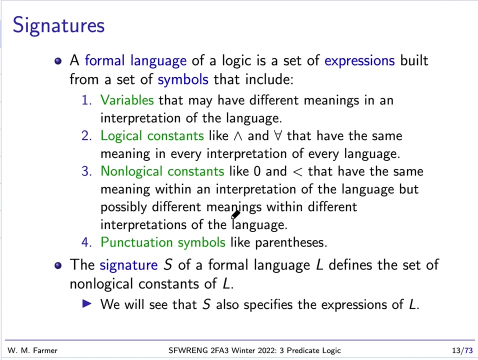 But this is an expression in subjunctive mood in which one is saying: we hope the king lives for a long time. So it is syntactically correct And it's It's also semantically correct, Okay. so if we have a formal language of a logic, we can think of this as a set of expressions built from a set of symbols. 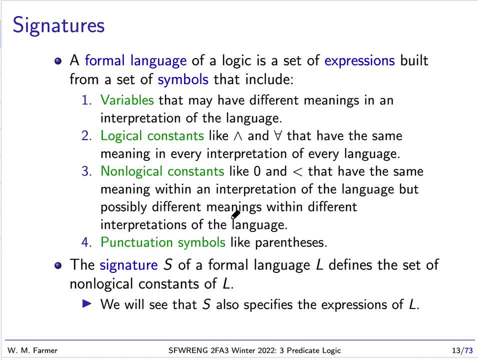 So we have a set of symbols and these symbols build expressions. From these symbols we build expressions. And there's four kinds of symbols. There are variables. A variable has a meaning which can vary in an interpretation of the language. So if we're thinking of the language as talking about something, the variable can take on different meanings. 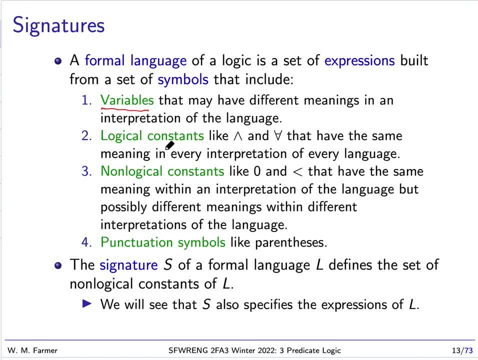 So if we have a variable for natural numbers, we can think of that variable could be 2,, it could be 5,, it could be 6, and so forth. So those are variables. Now, a logical constant is a symbol that has the same meaning in an interpretation of the language. 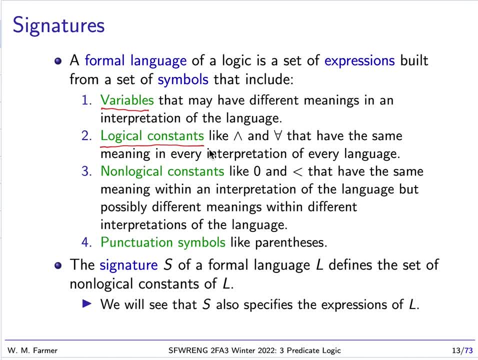 And it has the same meaning in every interpretation. So the meaning is completely fixed. A non-logical constant is a symbol whose meaning is fixed in a particular interpretation of a language, but it could have different meanings in different interpretations. And finally, we have punctuation symbols like parentheses. 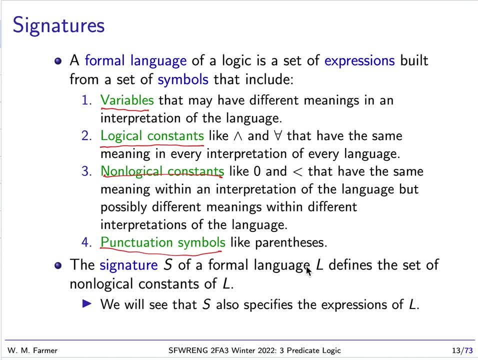 So a signature. So a signature defines the set of non-logical constants, These things, Constants which have a constant meaning in an interpretation, but they can have different meanings in different interpretations. And so a signature is a set of these non-logical constants and a signature specifies the expressions of the language. 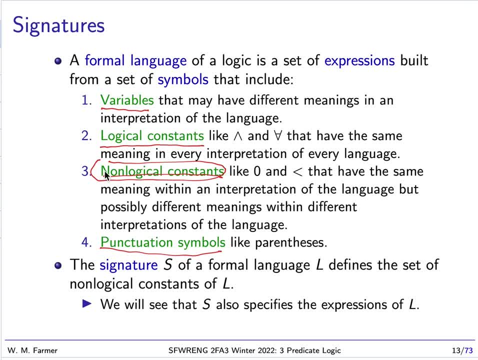 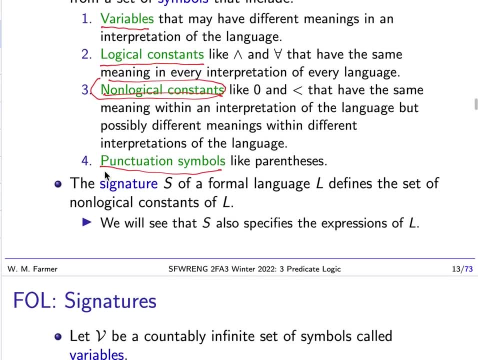 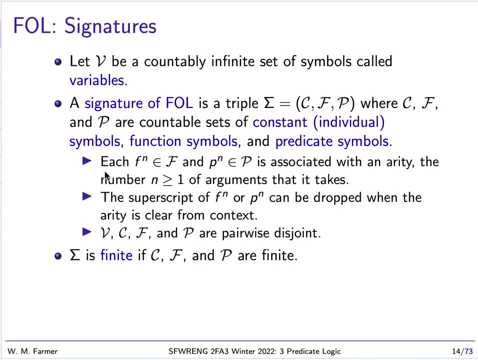 Or another way of thinking about this is: once we know what the signature is, we basically know the whole syntax of the language. So in first-order logic we have signatures that can be defined very simply. We'll start by saying that V. here is a set of symbols called variables. 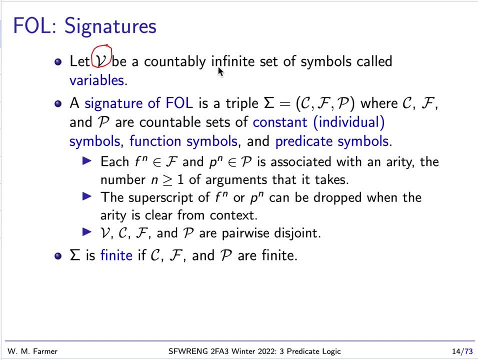 So we have some set of symbols called variables. It's countably infinite, which means that we are never going to run out of them. We always have an infinite number of variables that we can choose from, And our signature has three sets: Script C, script F and script P. 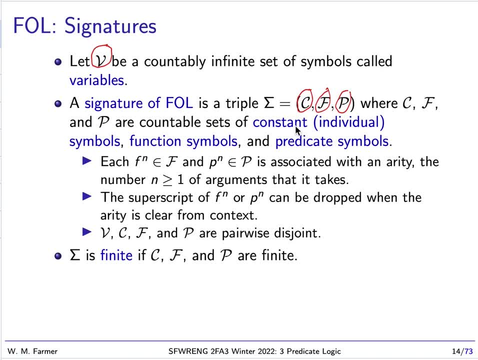 And these three sets correspond to sets of constants which are really individual constant symbols, function symbols and predicate symbols. So constant symbols, function symbols and predicate symbols. The function symbols and the predicate symbols: they come with an arity because these symbols are going to be applied to a certain number of arguments. 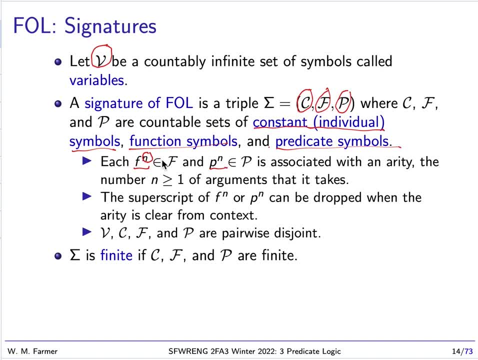 and that arity tells you how many arguments it can be applied to. So a function symbol is applied to a fixed number of arguments. That's its arity. And often this little superscript here is dropped when we know what it is And we assume that these sets are all parallelized as joint. 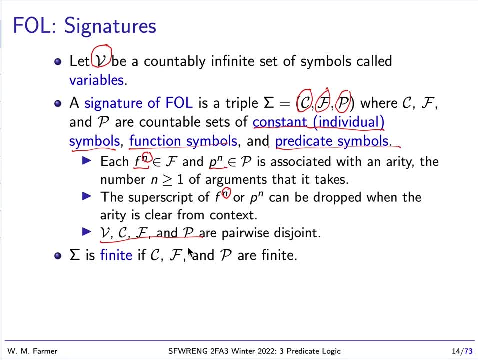 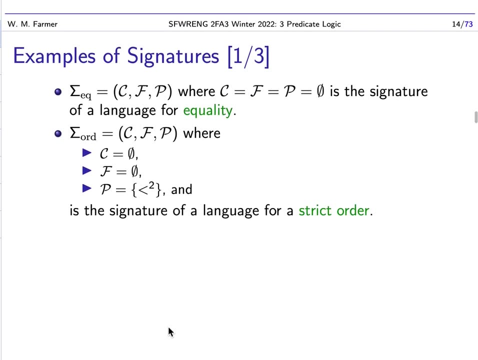 What that means is there's no symbol that occurs in more than one of these sets And we say: our triple sigma, our signature, is finite if each of the sets script C, script F and script P are finite. So let's look at some examples of signatures. 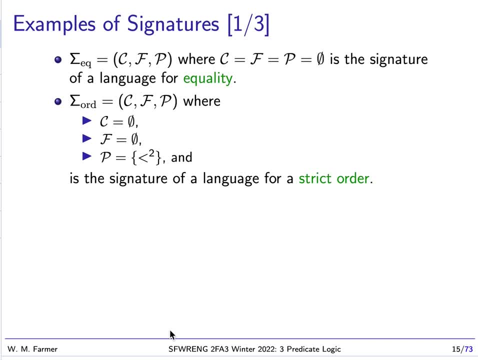 You can think of signatures as a set of symbols that talk about something. So the first signature is the- I'm going to call it the EQ signature. This is a language for equality And, in our logic, FOL- equality is built in. 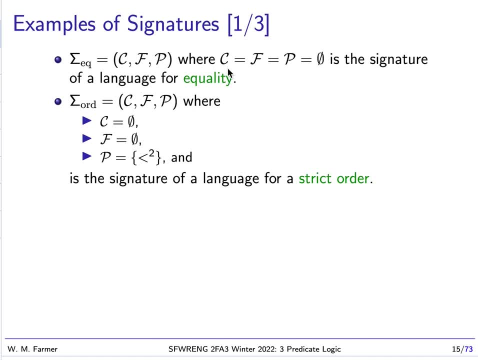 So we don't need any special symbols that talk about equality. For that reason, C, F and P are all the empty set. The next example is sigma ord. This is a language for talking about orders, So what we need is just a relation symbol less than. 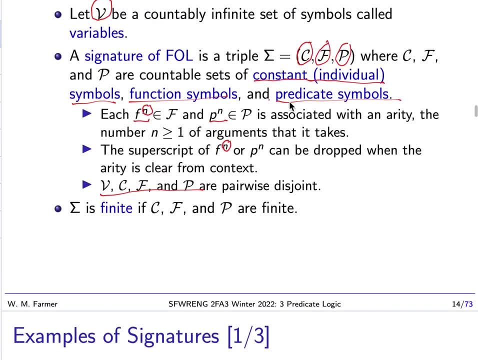 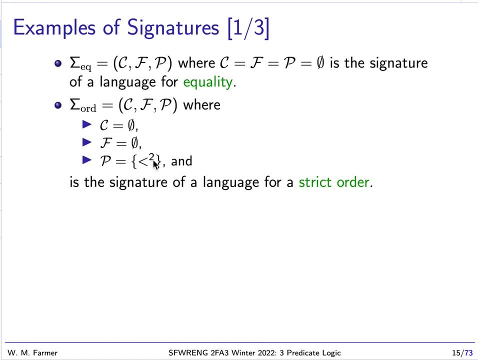 I said relation symbol. up here We these, actually I should have said predicate symbols. We're using predicate symbols to represent relations. So the difference between a relation and a predicate is: a relation is a set of ordered pairs. A predicate is a function that takes. I should say a relation is a set of ordered tuples. 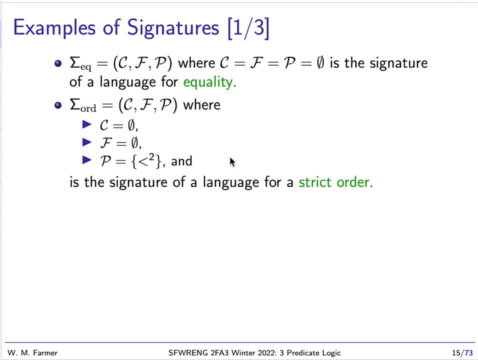 And a predicate takes a tuple and returns tuples. True or false, So they're essentially the same. So we need a binary predicate, a predicate with arity two to represent less than So. that's what this signature is for. It's for talking about strict order. 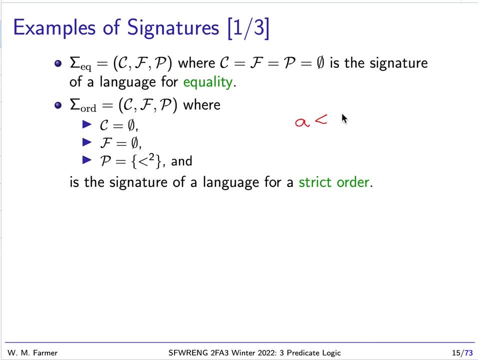 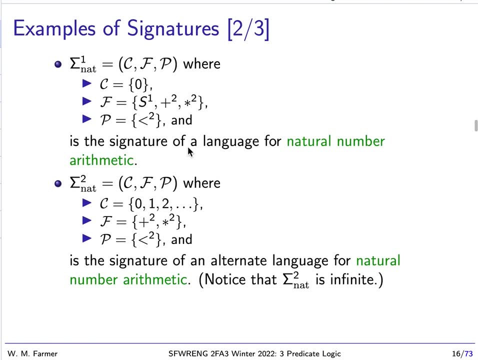 So we can write down statements like this: A is strictly less than B. Okay, so I have a couple more signatures. We have two signatures for nat, one and two, And in the first one we don't have any constant symbols, but we have three function symbols. 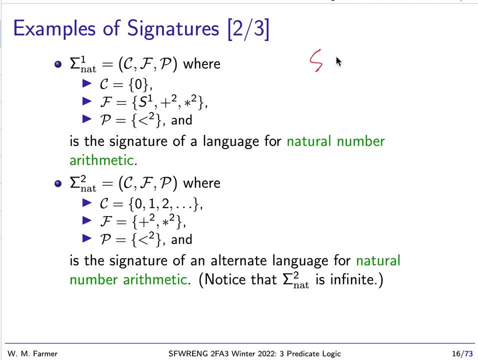 This is a symbol for successor. So, like the successor function, successor of two is three, Successor of 100 is 101, and so forth. And we have plus and minus And the successor function is unary. plus and minus are binary. 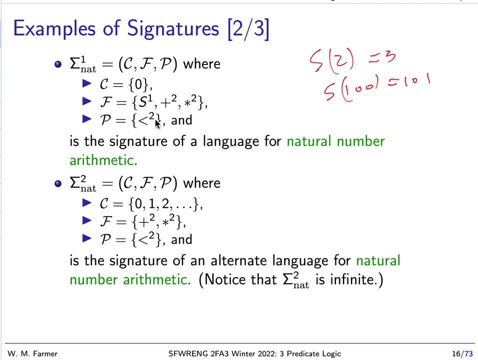 That's why we have these arities And we have less than which is binary, as we've seen before. So this is one signature for natural number arithmetic. Here's another one. In this case, we have an infinite number of constants: 0,, 1,, 2,, 3,, 4.. 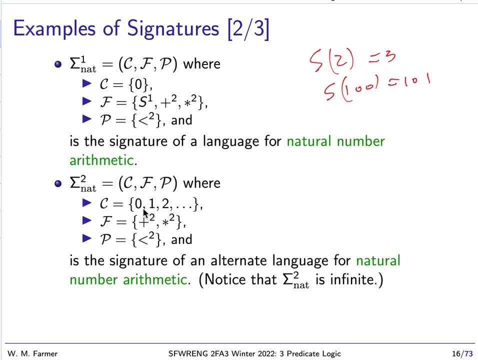 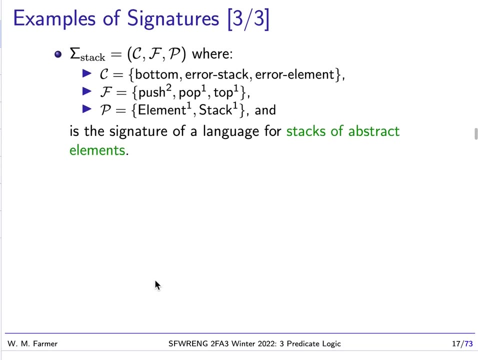 These are constant symbols And these are going to denote the natural numbers. And then we have plus and times and less than. And what's interesting about this signature? it is an infinite signature, because C is infinite. Okay, so we have one more signature to look at. 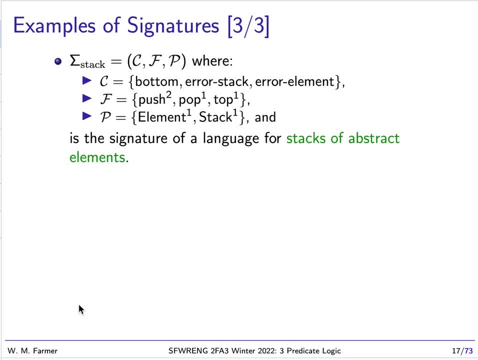 This is a signature for talking about stacks. And remember, with stacks we stack up something, So we think of it like this: We stack up things. So there's two kinds of individuals we have. We have stacks and we have the things we stack. 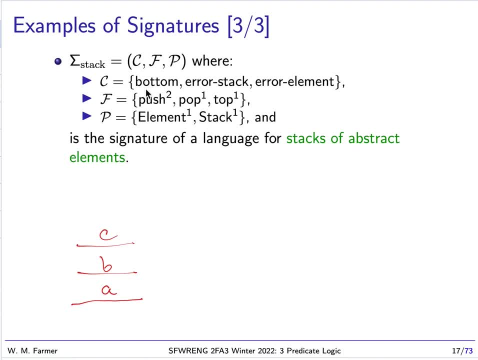 And so we need a language for talking about things, And so I'll look at our predicate symbols first. We need a predicate to tell us when an individual is an element, the thing we stack up, And we need one to tell us when we have a stack. 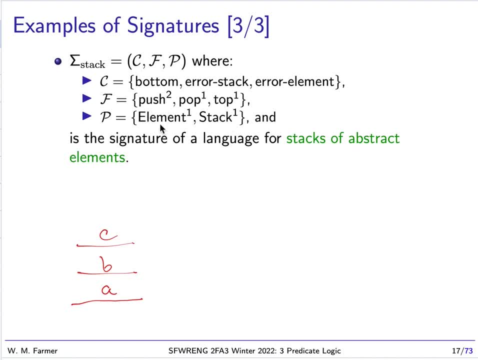 And we have functions, push. Push puts something else on our stack, And then we have pop. Pop takes off what's on top of the stack and gives us back a stack, And top gives us a stack. Pop gives us the top element of the stack. 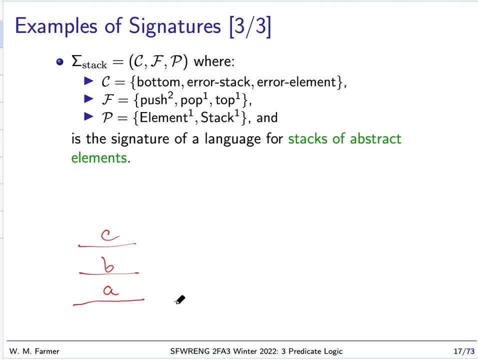 And then we have some constants. We have bottom- That's the starting point- a stack that has nothing on it. We have the air stack. The air stack is a stack that when we have, let's say, the empty stack and we pop it. 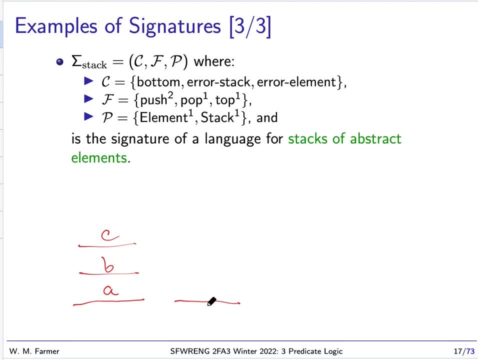 well, we can't pop the empty stack. There's nothing on it to pop, So we get an air stack And we have the air element. That's when we try to take the top value of an empty stack. There's no top value. 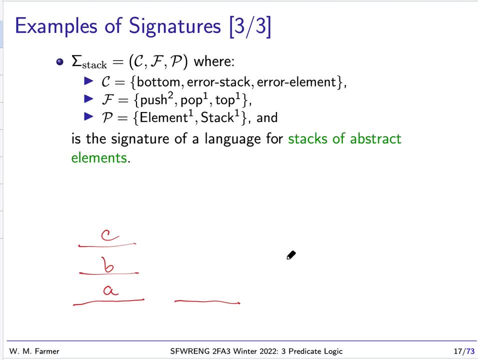 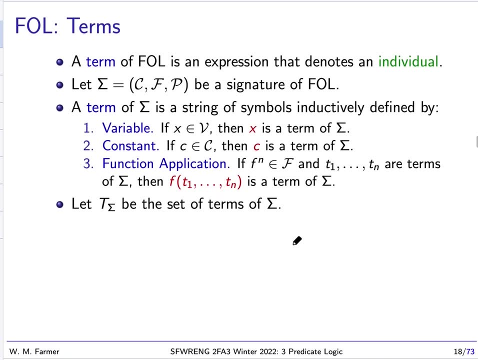 So we get the air element. So this is a signature for talking about abstract stacks of abstract elements. Okay, So now, once we have a signature- so let's say we have this signature sigma- now we can define terms, We can define the terms of this signature. 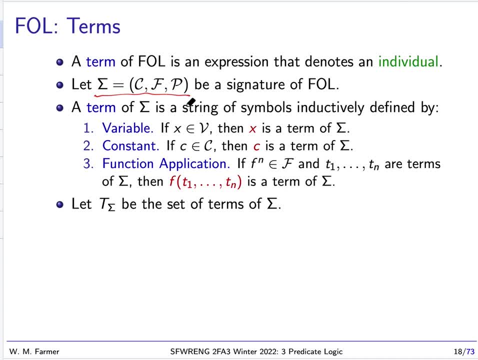 And a term is just an expression that denotes an individual And, remember, individuals are whatever you want to talk about. Individuals can be essentially anything, Depending on what we're concerned about. So a term of sigma is going to be a string of symbols inductively defined by the following statements: 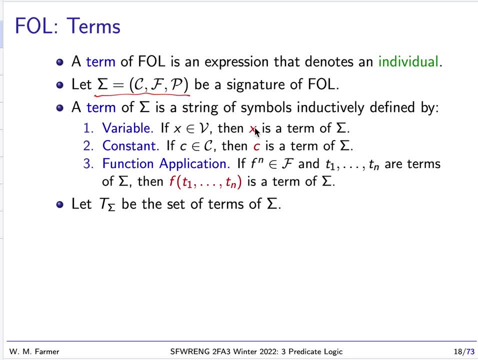 So the first says that if x is a variable, x is a term, So every variable is a term. If c is a constant, and that means a constant of our set of constant symbols, then c is a term of sigma, So every variable is a term of sigma. 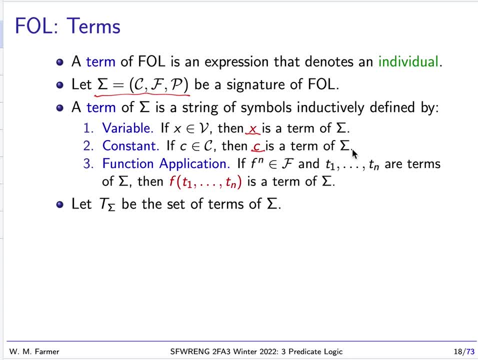 Every constant symbol in c is a term of sigma. And finally, if we have a function symbol of a or d, n and n terms of sigma, then the application of that function symbol to those n terms is a term of sigma. So there's just three ways of making terms. 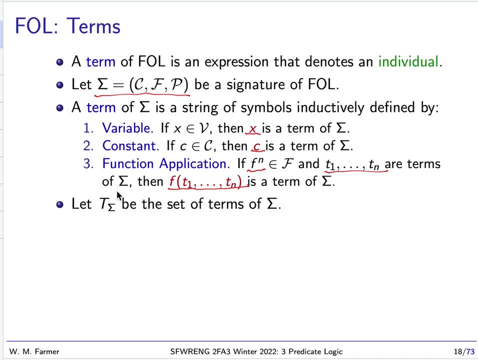 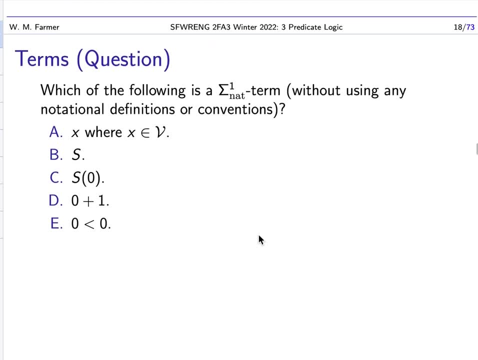 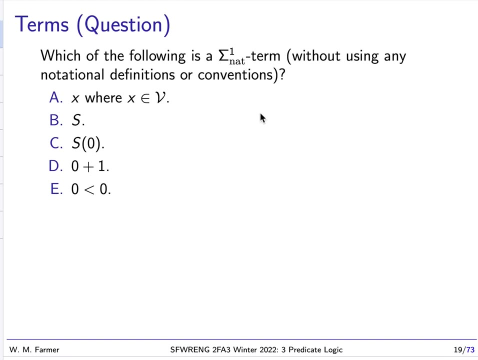 We have constants or variables, constants and function applications, And t-sub-sigma will be the set of all terms of sigma. Okay, so here's another question: Which of the following is a sigma-1-nat term? Remember sigma-1-nat. 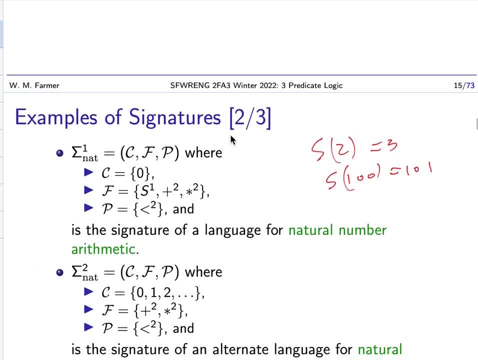 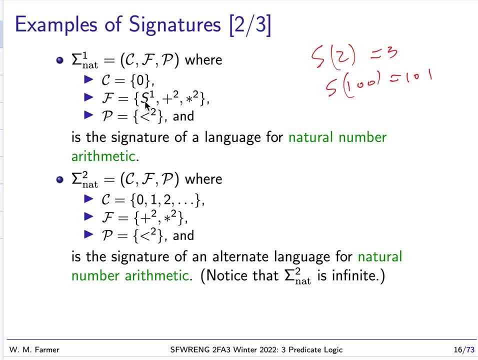 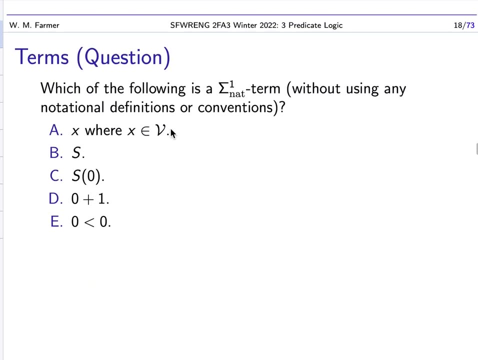 Well, we can just go back up and look at it to remind you. Here it is: In c we have 0.. In function symbols we have s-plus and times And predicate symbols we have less than Okay. so which of the following is a c-1-nat term? 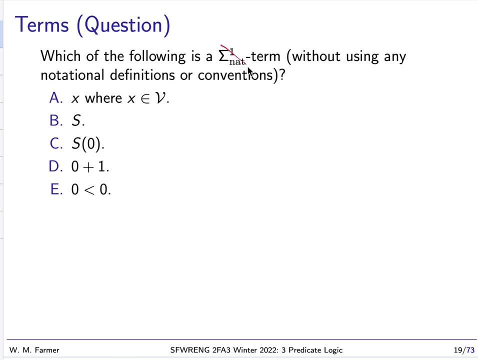 Actually the way I wrote. I should probably change this The way I was writing this. this is a term of c-1-nat And we're not using any notational definitions and conventions. We haven't talked about those yet. 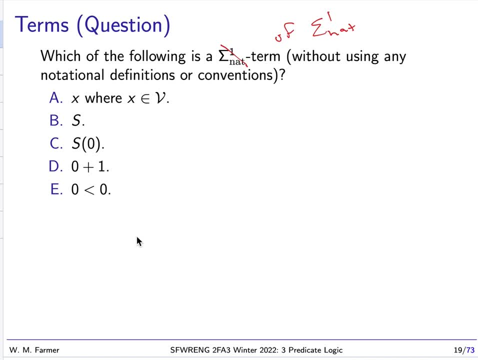 Take a moment, Think about which of these is a c-1-nat term. Okay, Okay, well, welcome back. Well, x is certainly 1. All variable symbols are terms for every signature. S is not a term. All s is is a function symbol. 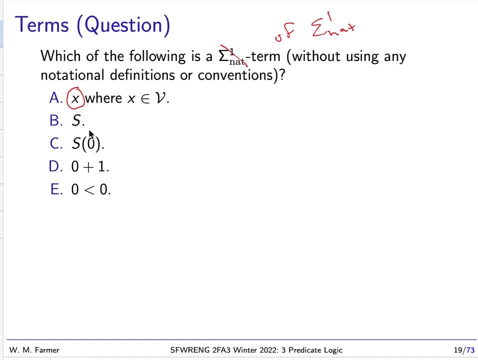 Function symbols need to be applied to things to be terms. This is a term because s is a function symbol of our signature and 0 is a constant symbol. This is not a term because it's not written in the right form. It's not a symbol. 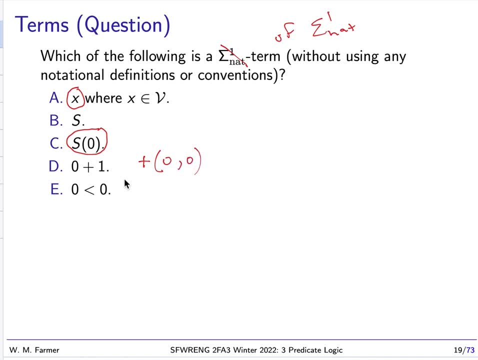 If it were written like this, then yes, this would be a term. This is not a term, because 1 is not a constant symbol of sigma-1-nat. It is a sigma-2-nat but not sigma-1-nat. 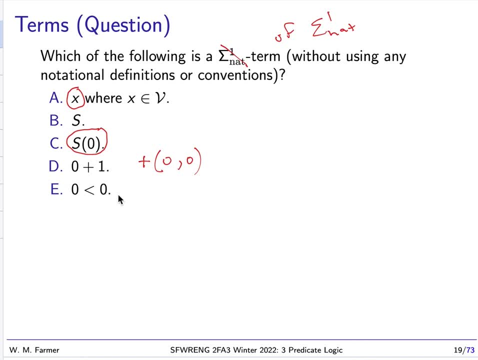 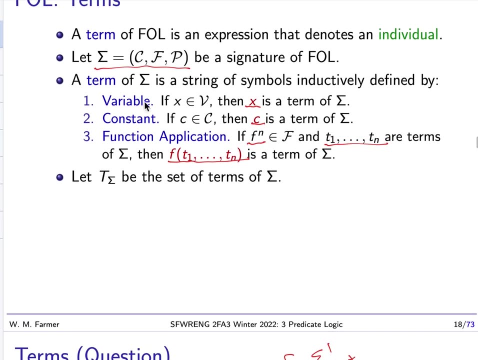 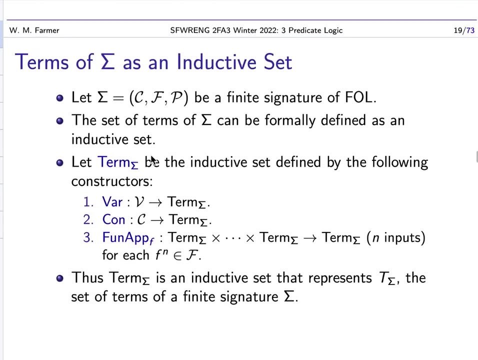 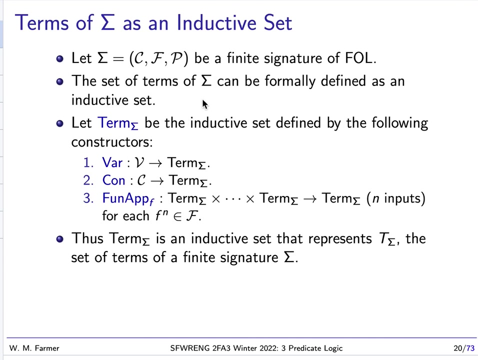 And this is not a term at all, because this is a predicate symbol. Remember, terms are variables, constants of function, application. They're not predicate applications. Now, the interesting thing about the terms: if we take the terms of sigma, we can define this as an inductive set where we have a constructor var. 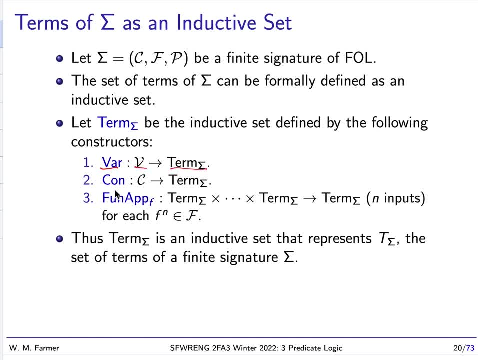 which takes a variable and gives back a term of sigma, Con, which takes a constant and gives back a term of sigma. And now, because function symbols take various arities, we need a constructor, one for each function symbol. And if that function symbol has arity n, it takes n terms. 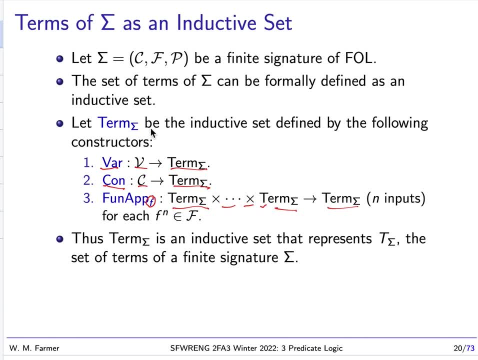 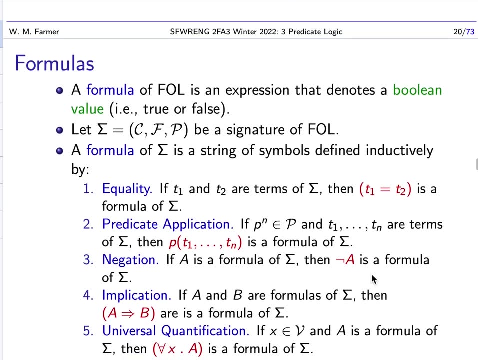 And gives back a term. So we can define term sigma as an inductive set And that inductive set, it represents the set of terms of sigma. Okay, so now we know what terms are. Let's move on to formulas. 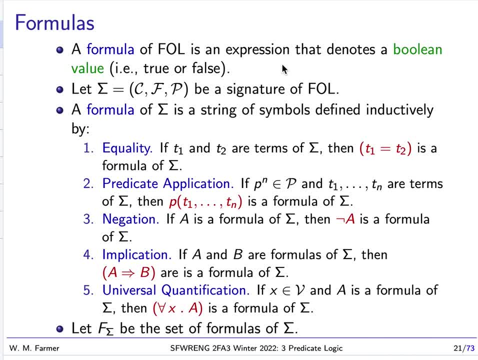 So a formula is an expression like a term, But remember, terms denote individuals, Formulas denote a Boolean value, either true or false. And so let's say we have a signature And a formula of this signature is a string of symbols defined inductively. 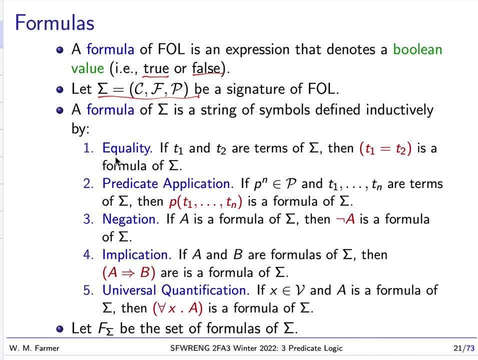 by the following five statements We can have equalities. So if we have two terms, we can put them together and form an equality. That is a formula of sigma. If we have a predicate symbol of arity, n and n, terms of sigma. 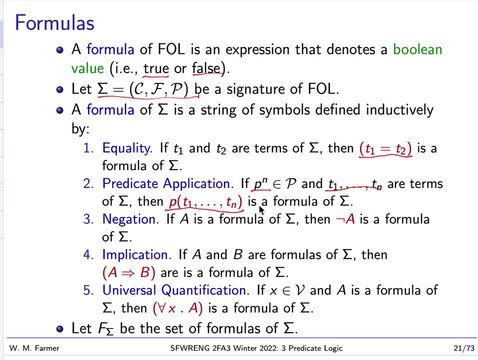 then the predicate symbol application to the n terms is a formula. Notice: predicate applications are formulas. Function symbol applications are terms. And now if a is a formula, then we get basically: non-a is a formula. If a and b are formulas, then a implies b is a formula. 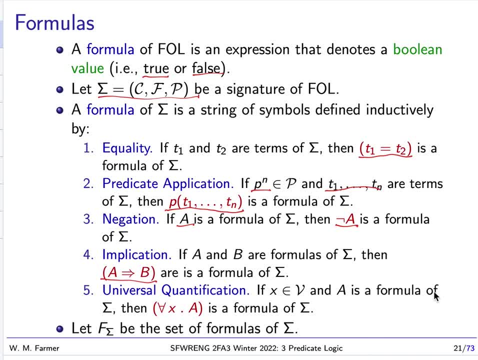 And if x is a variable and a is a formula of sigma, then for all x dot a is a formula. So we have five ways of constructing formulas: Equalities, predicate applications, negations, implications and universal quantification. 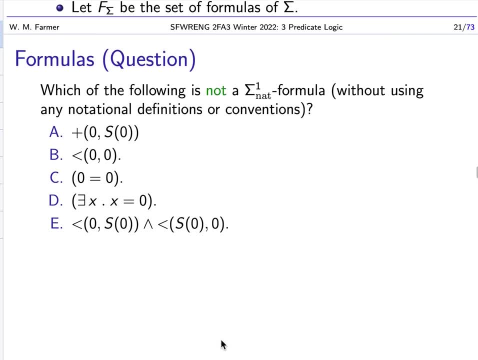 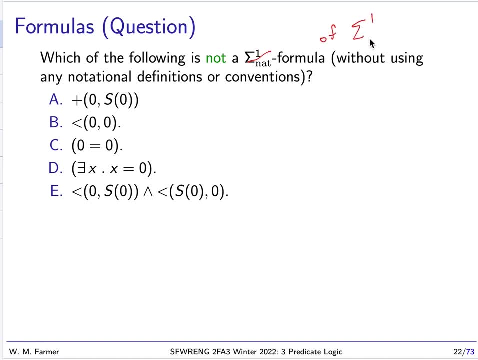 Okay, so let's take a moment. Here's another question. Again, I shouldn't have had this. I should have said: what is the formula to be consistent Formula of sigma 1, nat. So which of these is a formula of sigma 1, nat? 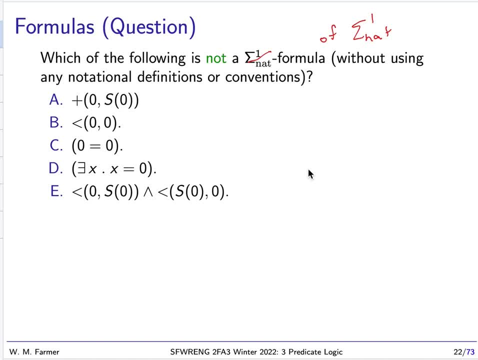 Or which of these is not a formula of sigma 1, nat. I'll give you a moment to think about that. Well, let's go through each of these. This is a function symbol, So this is clearly a term. 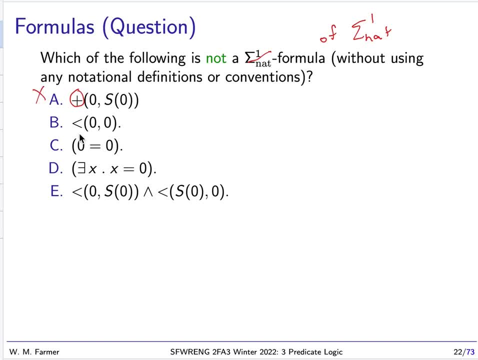 so it's not a formula. This is okay, because this is a predicate symbol applied to two terms. This is an equality. An equality is equals where on the left-hand side we have a term and the right-hand side we have a term. 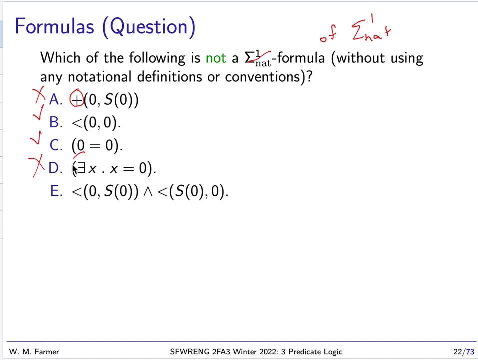 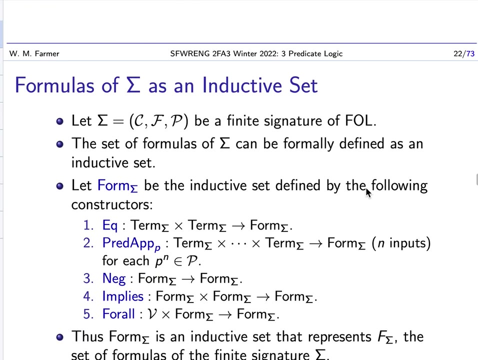 This is not a formula. We don't have this symbol, And likewise this is not. These are formulas, but the whole thing is not a formula because we don't have this symbol. So just B and C are formulas. Now, just the way we define what. 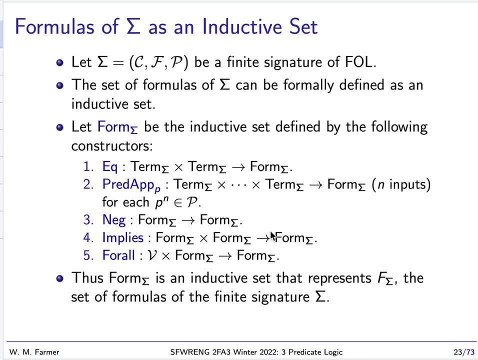 define the set of terms of a signature as an inductive set. we can define the set of formulas as an inductive set, So let sigma be a. I should say this is: We can do this when we have a finite signature. 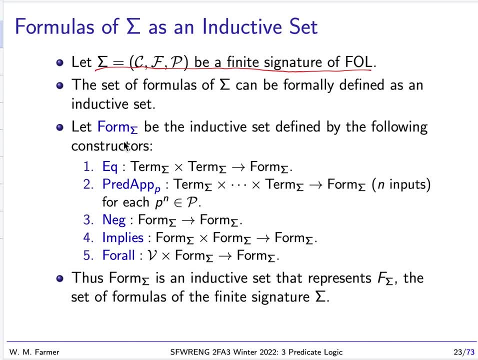 Let sigma be a finite signature. the set of terms of f allow And we'll define form sub-sigma and we'll have five constructors or five kinds of constructors: eq, eq, q, pred-app, P for each predicate symbol. 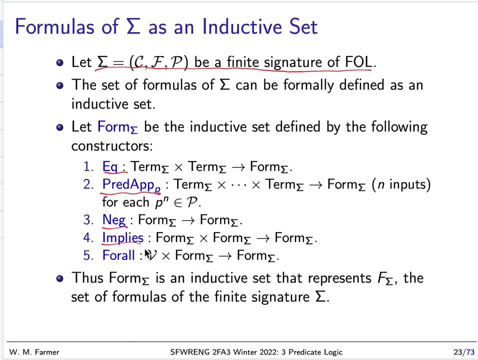 Remember we have only a finite number of neg implies and for all. So eq takes two terms and gives back a formula. Pred-app takes n terms terms, depending on the arity of the predicate symbol. gives back a formula, Negation takes. 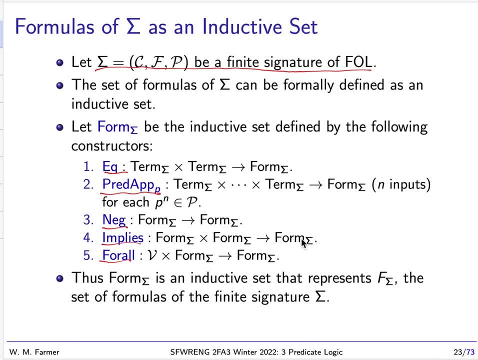 one formula and gives back a formula. Applies, takes two formulas and gives back a formula. And for all, takes a variable and a formula and gives back a formula. So this inductive set defined by these five groups of constructors represents the formulas of our signature sigma. 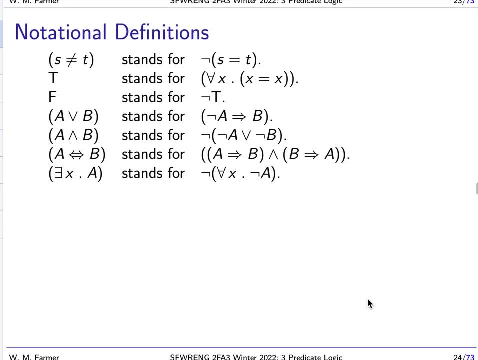 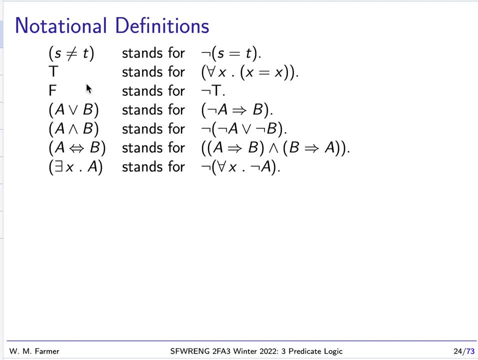 Okay, so we would like to make some notational definitions, And these notational definitions are in this case. you can think of them as abbreviations, but they're a more convenient way of writing down something you want to say. So, instead of saying not s equals t, we can say s does not equal. 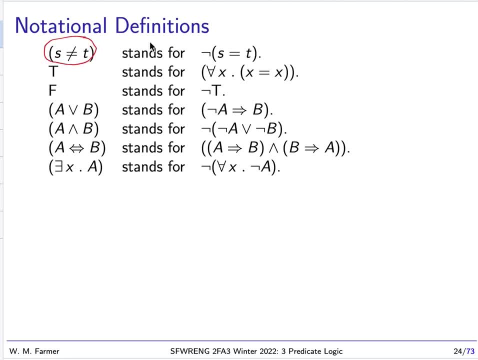 t. So this expression really stands for this expression. The one on the right is the official version, the one on the left is the convenient version. So t will stand for a true formula, and one of the truest formulas is for all x. x equals t. 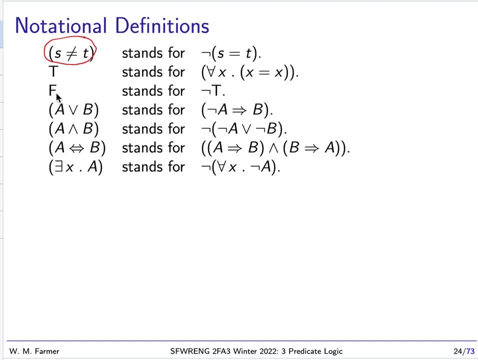 So we can say that s equals x And we need a. f stands for a false formula, not t, And we want to introduce or and and This is called biconditional or logical equivalence. Or is going to be. we have to define using not and implies. It's going to be not a implies. 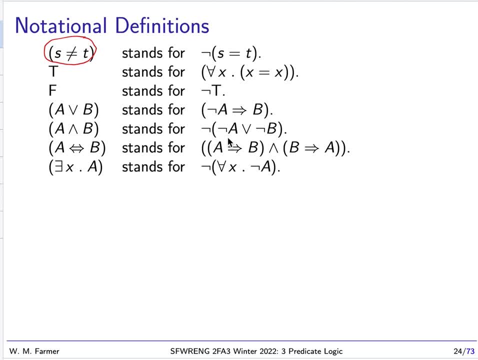 b And is going to be not the. not the disjunction of not. And this is going to be not the disjunction of not a and not b. Remember, if you remember, De Morgan's laws, if we push in the negation, 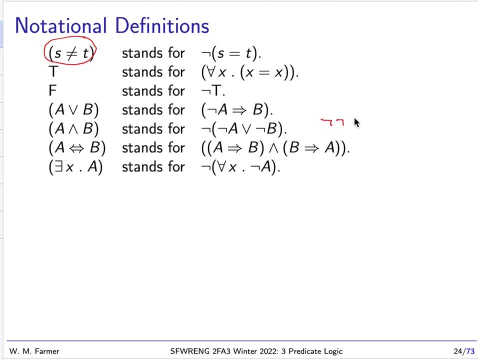 into this disjunction. we get not, not a, And then we flip this and not not b, which is equivalent to a and b is what we have here, And logical equivalence or this, like I said, could be called biconditional. 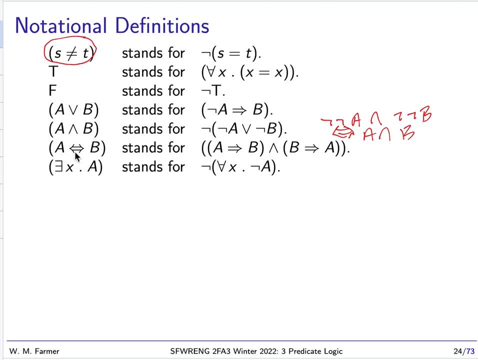 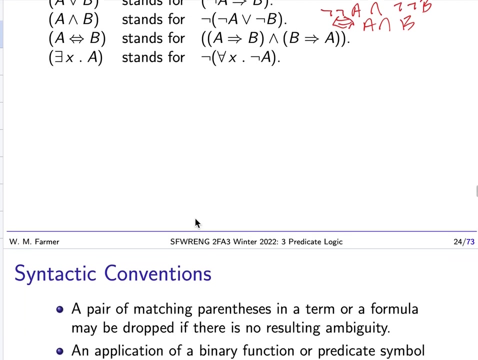 It's sometimes called bi biimplication. It's also called if and only if. This is just going to be: a implies b and b implies a And existential quantification. that stands for not for all, x, not a. So we're going to freely use these notational definitions because they are convenient. 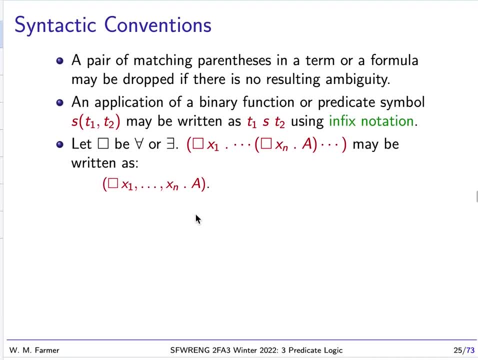 We're also going to use some syntactic conventions, Okay, Okay, All right, Let's machine some of these guilt-saving migrations- And these are also called notational conventions. And so the first one is: we can drop pairs of matching parentheses in a term or a formula when there's no resulting ambiguity. So for 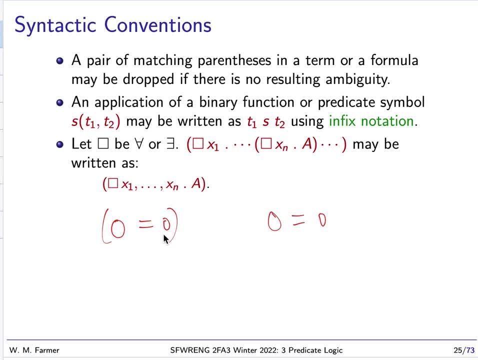 instance, if we had zero equals 0, we can write that just as zero equals, But the parentheses don't really aren't really necessary if we had something like this- this is the second notational convention. If we had something like this: 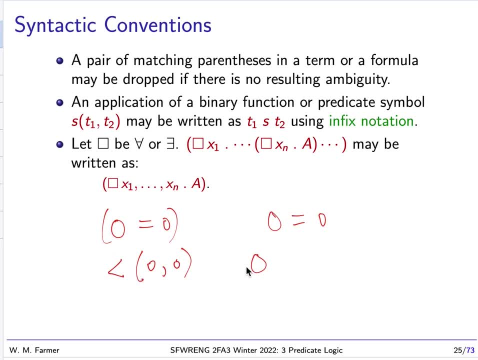 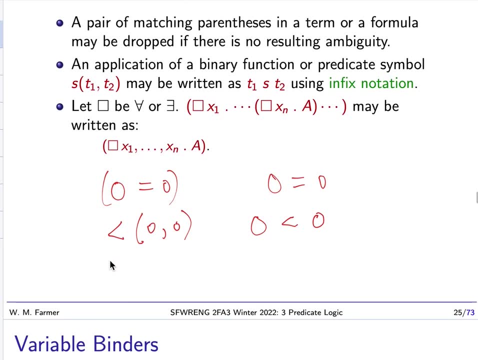 we can write it, because this is a binary predicate symbol. we can write it in an infix format, Because that's what people normally do. And the last convention is: if we had something like for all x dot. for all y dot- x is less than y, and I'm using the second convention here- we could write: 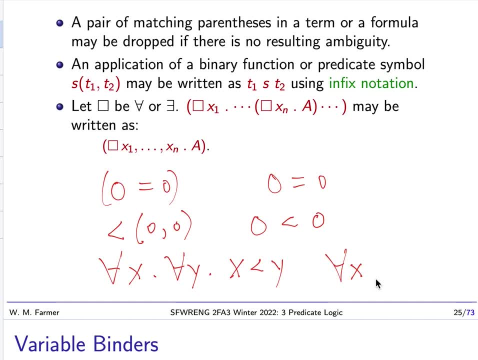 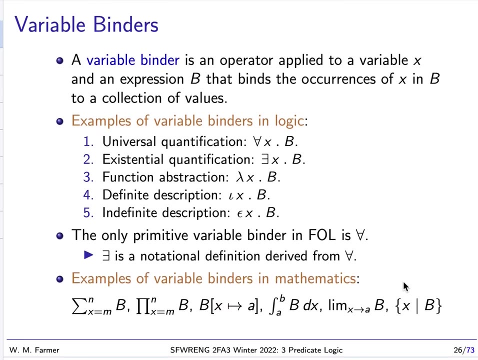 that, simply, as for all x comma, y dot x is less than y. Okay, so we're going to stop here. Next time we're going to talk about variable binders, So I'll see you all then.